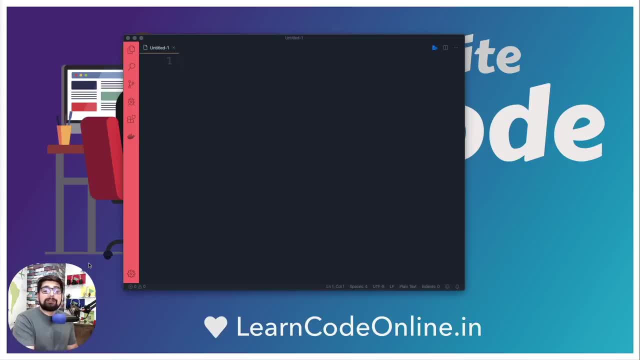 that functional programming is, moreover, of writing style of code, So it's majorly independent of programming language, But there are some programming language which is supporting it to its at its best. Some are not. So there are a couple of concepts that you need to understand. 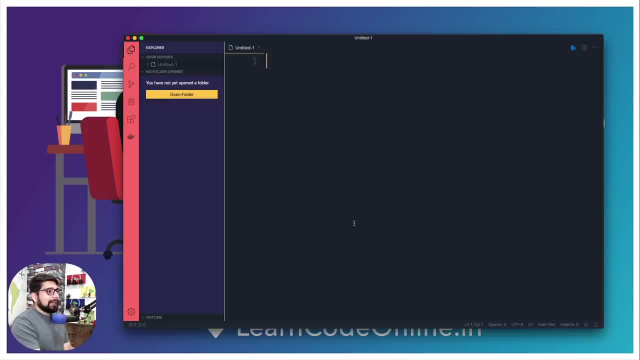 Let me explain this. This is just simply a VS code And I'm not going to be running any code. I'm going to just explain these syntax using the help of code. So let's just say we got a score and you are playing on to some great level. you got a score of 456.. 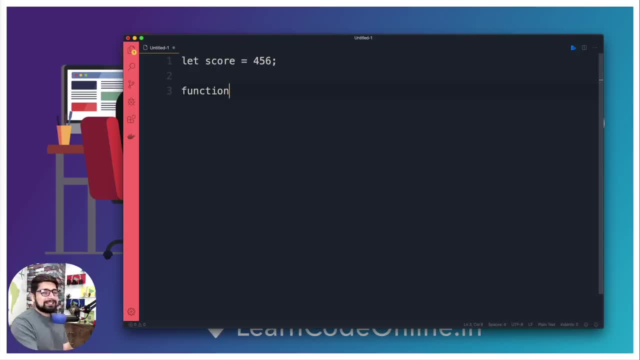 Now, on that, let's just say you have a function. Again, this is not really a core function, it's just the gist of how function usually looks like. So we're going to simply say that at this exact stage, you have done something so that we want to add a bonus up here, What you can do up here. 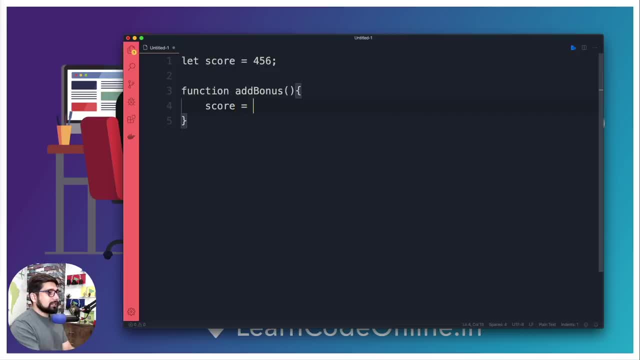 you can simply call this up here, simply say score is going to be equals to score plus, and you just add some number like 45. And finally you just go ahead and return score. Now don't yell at me by saying, hey, you should say this: dot score. 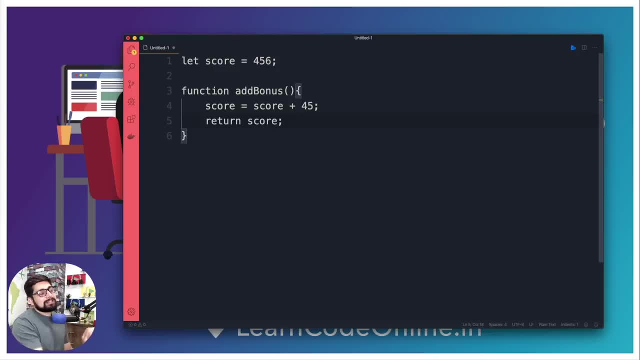 It's, moreover, about understanding the concept, not exactly pinpointing the stuff. So this is all okay, but this is not really much of an acceptable thing in functional programming, And functional programming, you're going to notice that these things don't happen. moreover, a functional 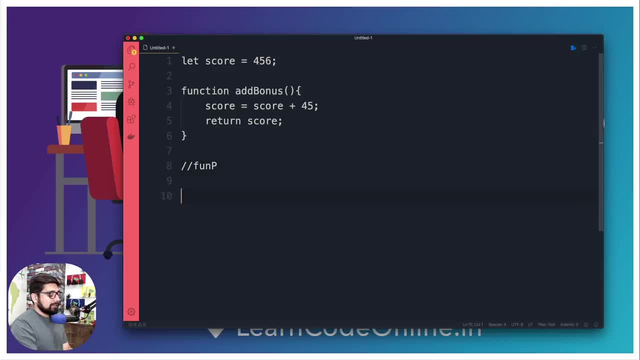 If I write this into a functional programming way, I would write it in a bit different manner. I would write the same function like this And I'm going to simply say that, hey, this is my function, again, add bonus And this is going to take a parameter. 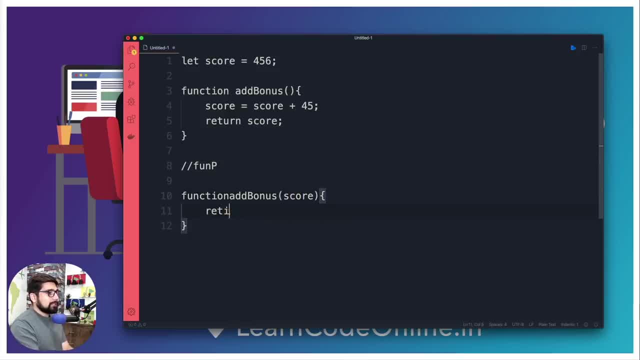 Score And what we're going to do now. here we are going to simply just hit return and we're going to simply say, whatever the bonus or whatever the score we have got, we just want to add. let's just say, 45 on to add. 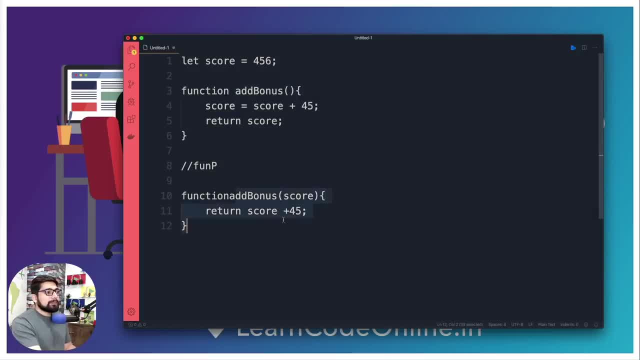 Now, there's a huge difference between this piece of code and this piece of code. No, it's not much shorter. You can also make it a shorter like this, but that's not the point. In the functional programming, we keep our functions and data totally separate. 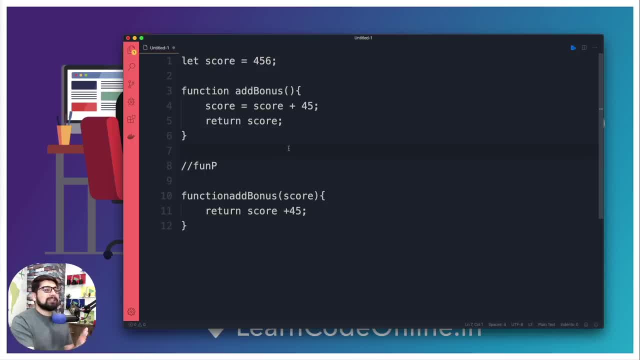 So that's the step number one. This is an unspoken rule in the functional way so that keep your data and keep your functional totally separate. While debugging this piece of code is much easier to debug because it is not referring to any global variable which might be causing the issue. 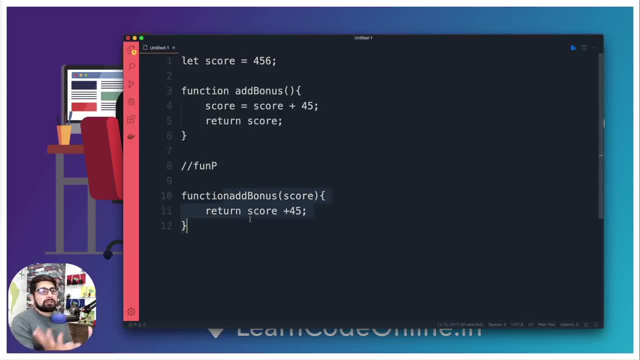 This is, moreover, like self intake function, which just runs on its own, And it's also not much, very dependent on what kind of data you're passing, whether it's a score, or maybe it's a life. whatever it is, it's just going to add 45 to it. 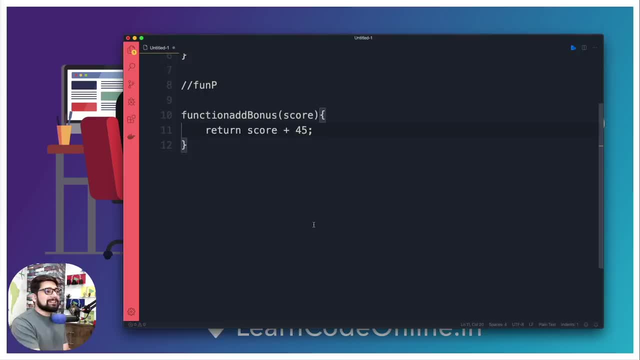 So that's the basic gist of it. So that's the one thing: Keep your data and keep your functions totally separate. So that's one thing. Now, again, one another thing is actually state change. So this is state change, is, if I can write that this is state change is a very interesting thing. 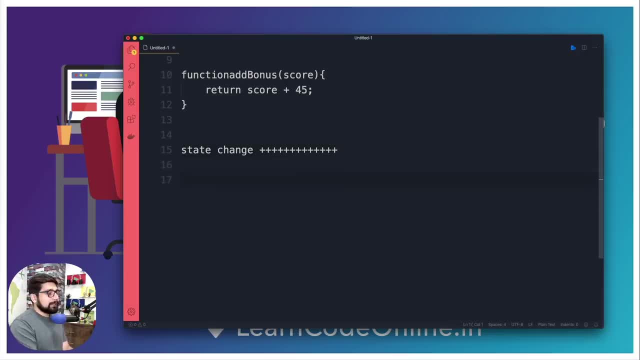 And it's a bit difficult to understand for beginners, but I'm going to try my best. These examples will just simplify like ridiculous level. So it says that you should not change the state much often. as much as you can avoid it, Just do it. For example, I am Hitesh. 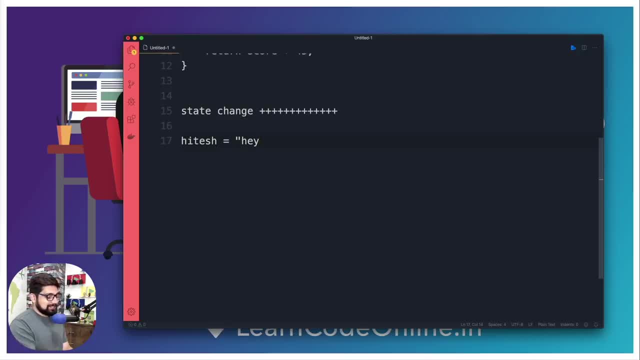 And I say let's just say hey, a lot, which is true. And then later on I realized that this variable should not say hey, it should say something like hey there. And then I realized the same variable should say something like this: 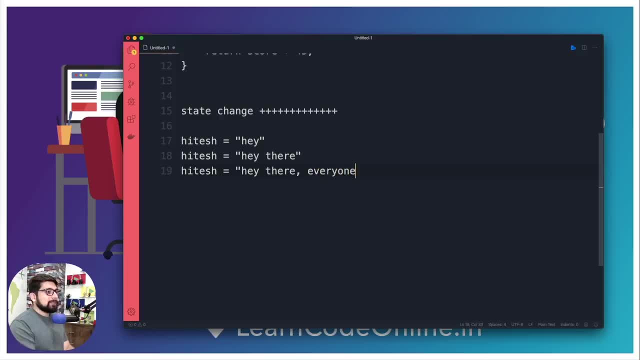 Hey there, And then everyone. So there is nothing wrong in this style of code. We are just having a variable and this variable is getting updated all the time. Now, keeping the track of this state is actually a bit tricky To understand. this one, 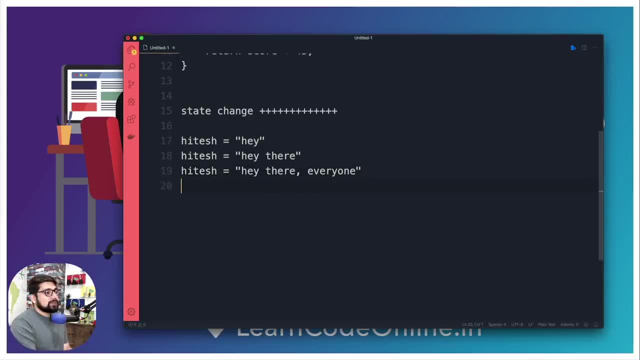 So in functional programming style, we actually don't reuse this variable much often, We don't change it much often. In fact, what we do is, let's just say, Hitesh says hey, and then we want to update this somehow. 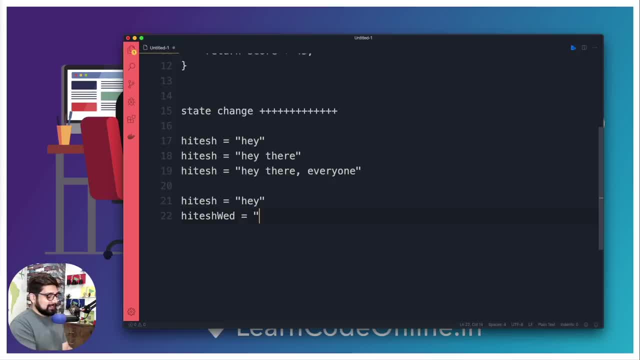 So we're going to say: Hitesh on Wednesday says hey there, If I can write it, hey there. And Hitesh on Saturday says hey there again, Come on, Hey there everyone. So this is, moreover, like a functional style. 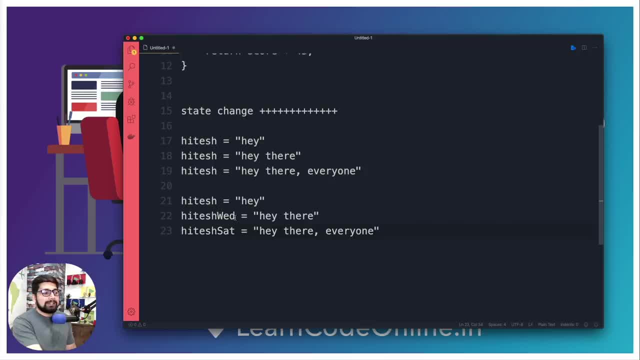 You don't update the same variable. In fact, it is okay to redeclare or kind of a newly declared again available with some more modification, so that it's much more clear, and it's okay for us. So this thing is pretty common of the don't change your state and mutability, mutability. 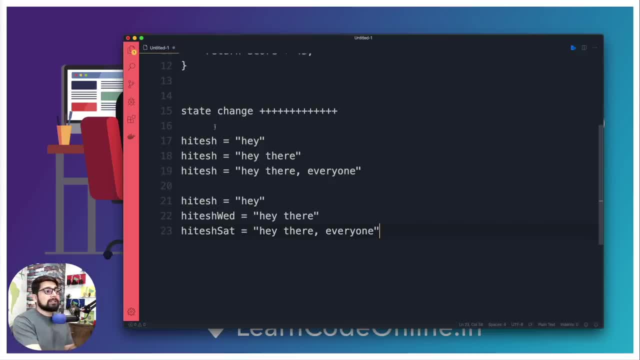 This is common thing in the functional programming. Again, the rule of thumb is that make sure you don't really update the same variable again and again. You instead declare more of them. Now coming up onto the last part, which is very funny and pretty interesting as well. 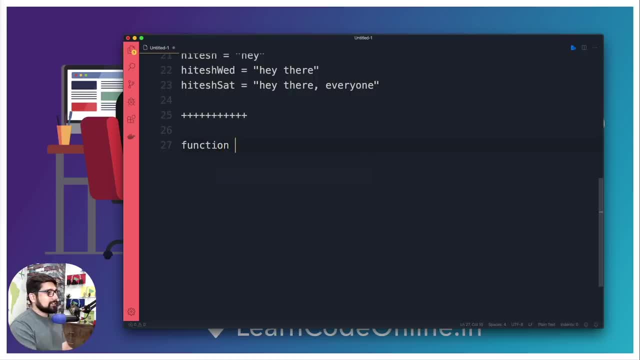 So in this, what they say is something like this: function or functions are treated as a first class. Okay, This is a bit of a bit difficult statement to understand for beginners, but I'm going to make it absolutely ridiculously simple. So let's just say we have a const with H and it is storing 45.. 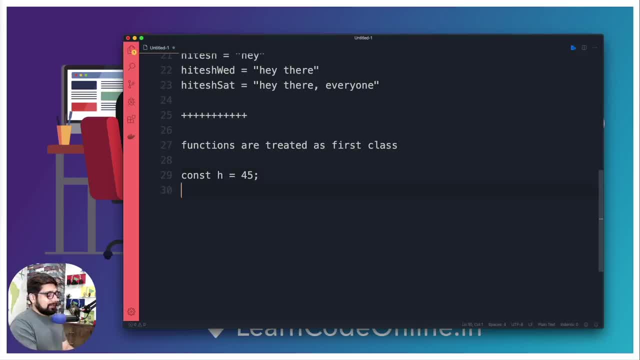 I don't know. I don't know why I'm always using 45,, but that's it. And we also have got a variable which is name in your language. However you define it, that's okay. And if I just say this variable is a page, that's okay. 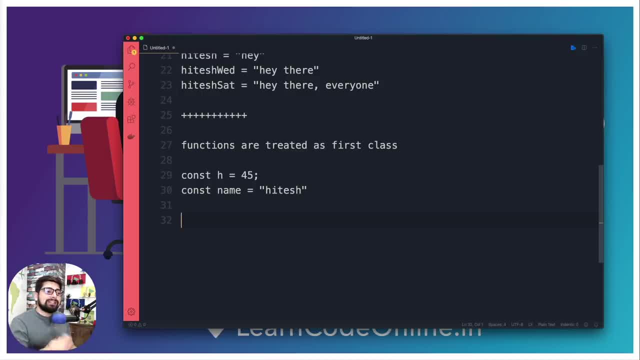 But what functional programming says that the way you are treating your numbers and string and you are throwing them around anywhere, like you can declare them in a variable, you can pass them in a function, you can return them in a function, The same kind of treatment should be given to the functions as well. 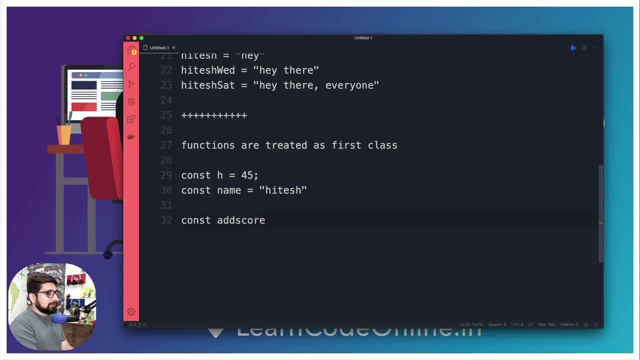 So we can simply say const: Add a score, something like that: add score, And that can also be a simple function. whatever you want to do inside that, That should be the case. I want to. I want to say this: 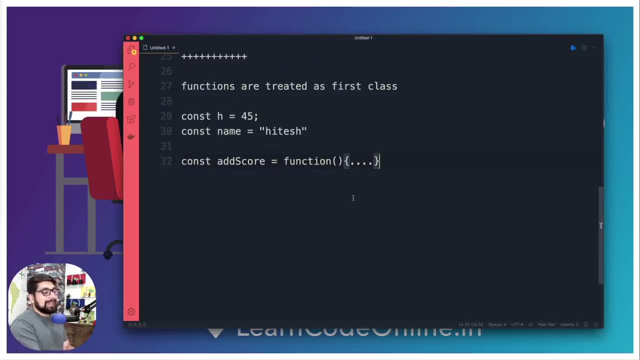 So this is how the function should look like in a functional programming. It can be, it should be able to store functions into any variable. And not only that, if let's just say you have a method which says: say hello, and this is our method in here. 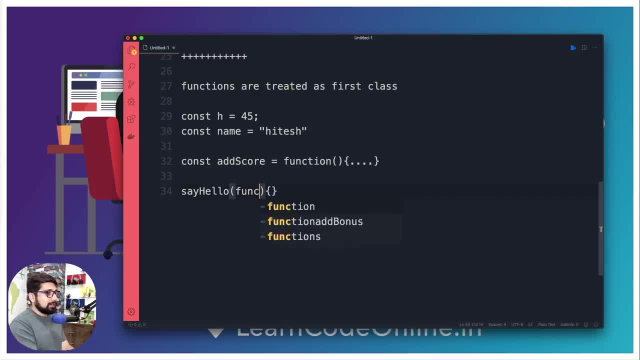 Also, you should be able to accept function as a parameter, So I can simply say a function and then simply say, like this, whatever you want to say- or maybe a reference would be a better example, but this actually makes things simple and easy.